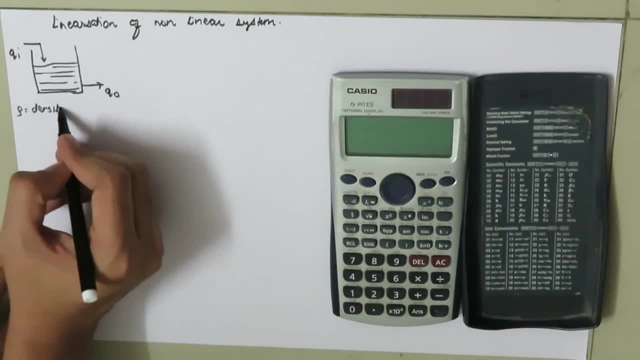 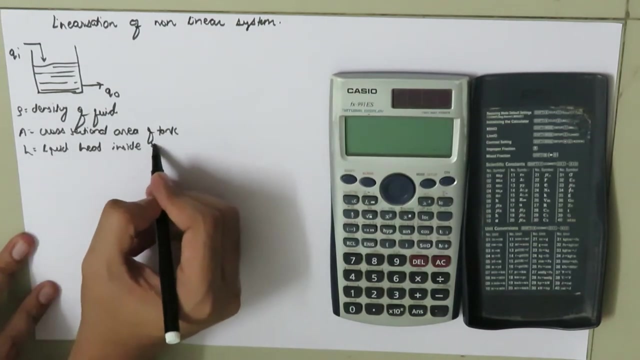 If rho is the density of fluid and A is the cross-sectional. So this is the area of tank, H is the liquid head inside the tank And the outlet volumetric flow rate is related to C times root H Here, as the outlet volumetric flow rate is expressed in the non-linear term. so we are going to linearize this expression. 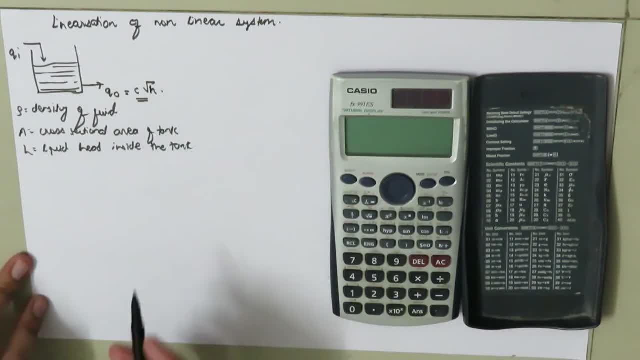 So here, as the outlet volumetric flow rate is expressed in the non-linear term. so we are going to linearize this expression. So if take the mass balance on this tank so we get mass flow rate in should be equal to mass flow out plus accumulation. 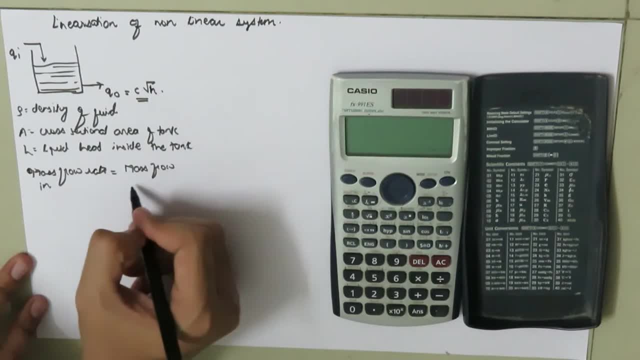 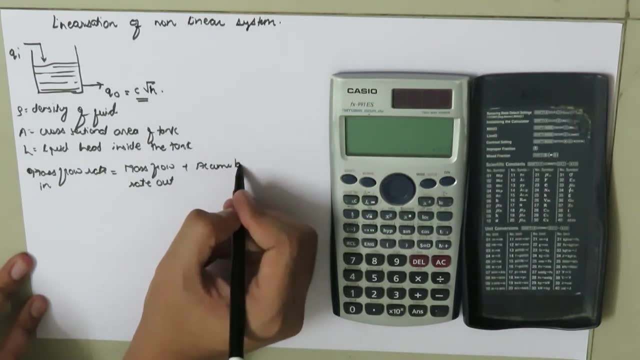 So if take the mass balance on this tank, so we get mass flow out plus accumulation. So here, as the outlet volumetric flow rate is expressed in the non-linear term, so we are going to linearize this expression. So we are going to linearize this expression. 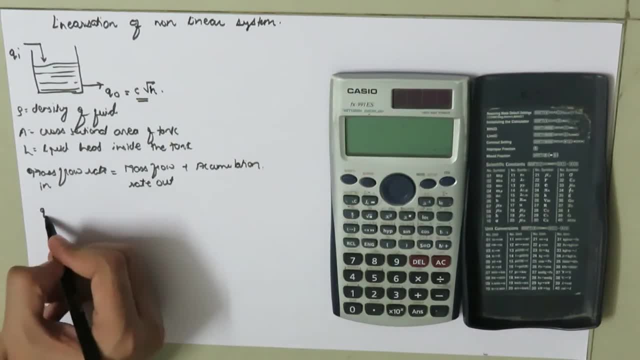 this expression in the mathematical form. so this will be Q I times Rho and this is Q O times Rho plus D over DT of a Rho H. let's check the dimensioning balance of this equation. so here, if it is in meter cube per second, the volumetric fluid. 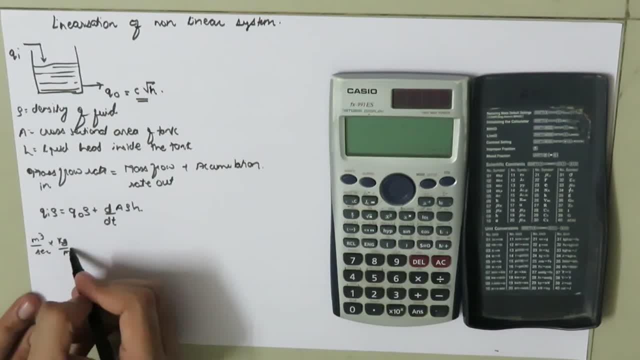 times the density is in kg per meter cube, so this is kg per second. okay, then this is correct and if you check the dimensions of this term, so this will be: A is in meter square, density is in kg per meter cube, height is in meter and divided by DT in second if you take. so this is also in kg per second. so, in fact, 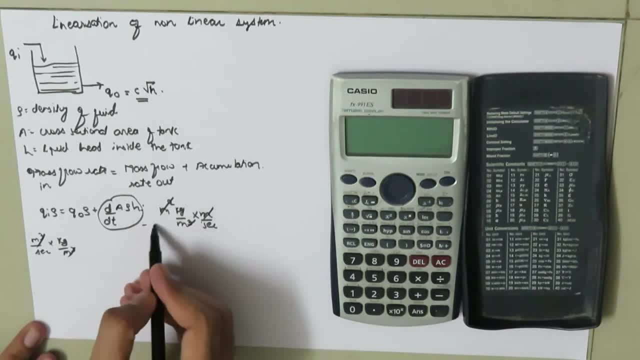 our mass balance is correct, so let's call this equation number one. now we are going to assume that the density of the fluid is constant, so Q I will be equal to Q O. let's write this: Rho O plus Rho times D by DT of a H, we can take the density common and it. 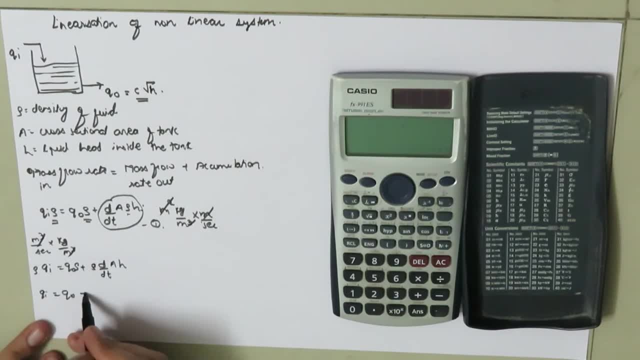 eventually get cancels. so Q I will be equal to Q O plus, if you take, the cross-sectional area of this tank is also constant, so this should be out of sign. so this will be a times D by DT of H. let's call this equation number two. 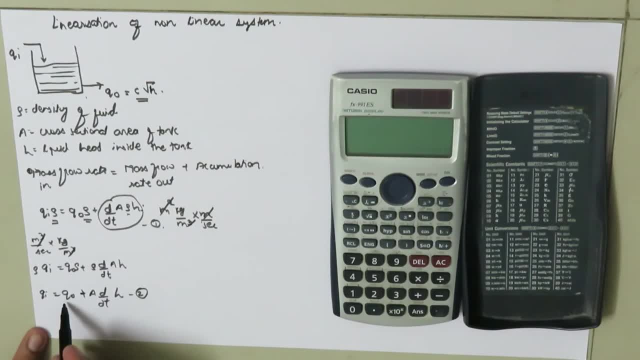 and now we know that our outlet volumetric flow rate is related to C times root H. so Q I will be equal to C root H plus a times D by DT of H. let's call this equation number three. and now in the case of steady state. so 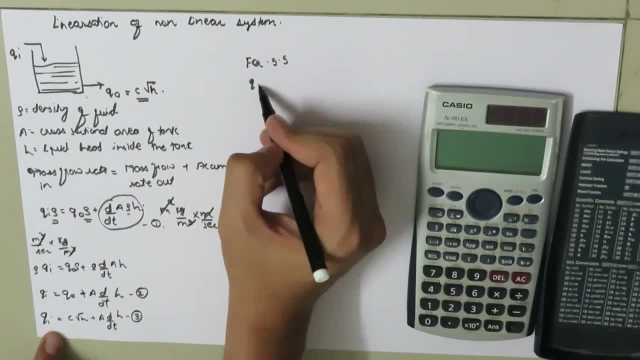 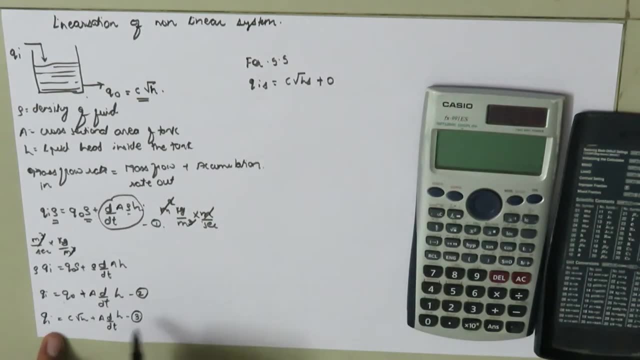 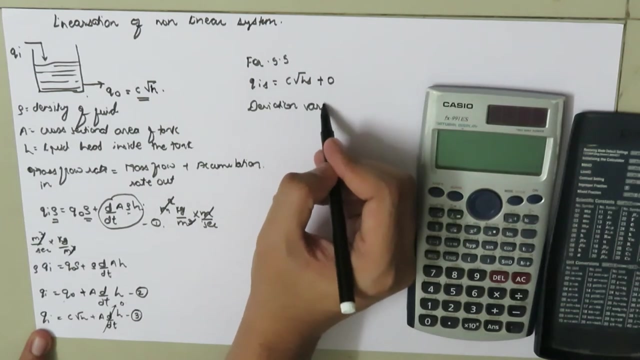 for steady state, Q R S will be equal to C root HS plus zero, because in this, in the steady state, this term will eventually chapter to zero. and now, if we introduce our division variable, so introducing our division variable, so if Q R minus Q is capital, Q for the når Q. Professor, I have a phone number and you want to start a one- rain number in this equation number into drop Player. so I have a friend number here, 0 here also and you can start same, so at any point you sprint one error to the end. so in terms of Stc, let's create the historic start using this equation number so that Les Q or a winnerstep, one zero after every agreement. 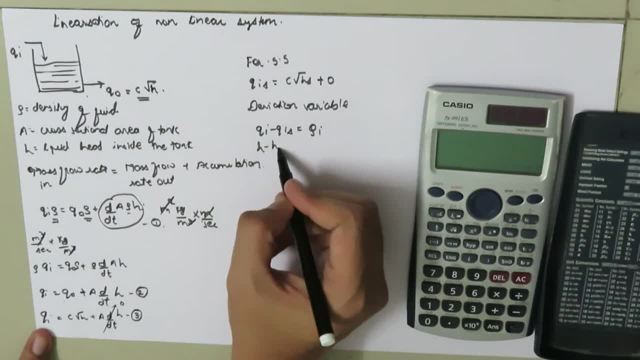 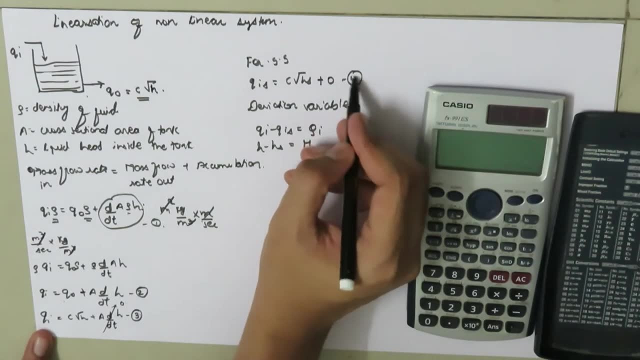 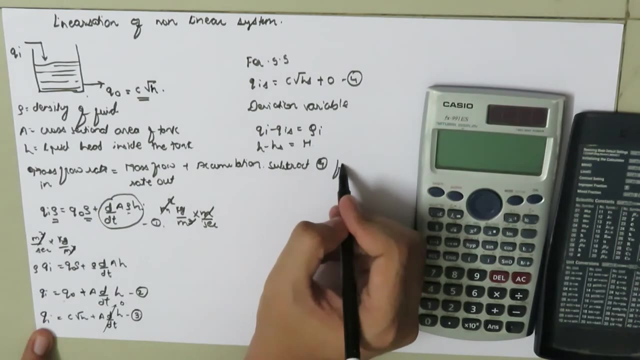 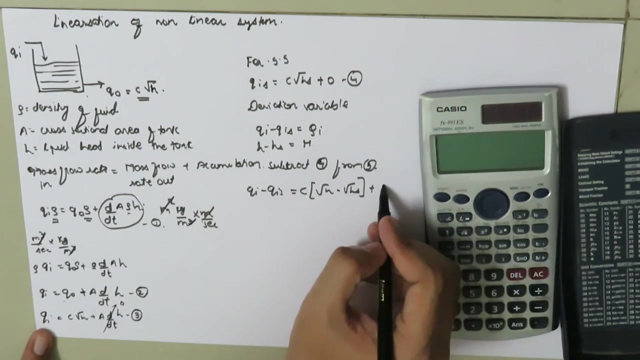 and our H minus H s is equal to capital H and that's called the equation number four. if we subtract equation number four from three, then this will be Q I minus Q I s. that should be equal to C times root s minus root H s, plus a times T by DT of. 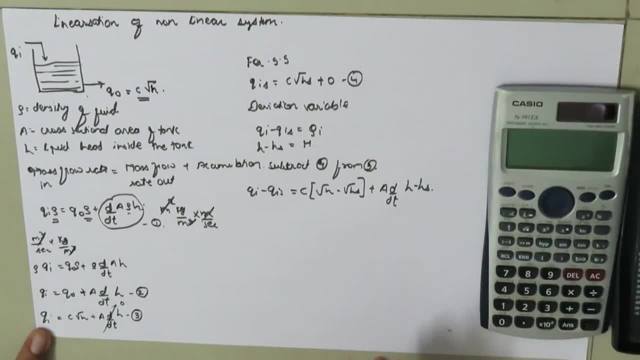 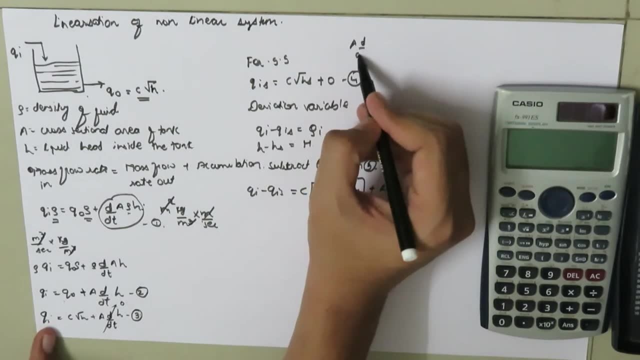 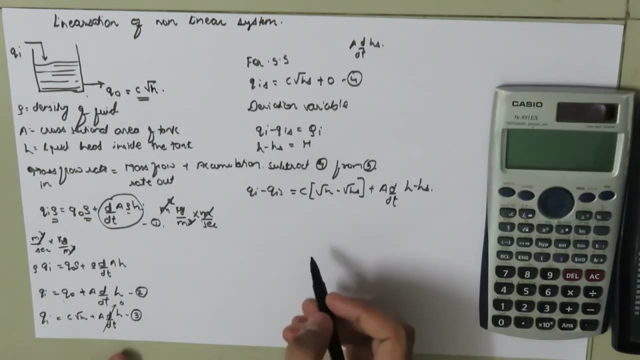 H minus H s, because at this steady state we are going to assume that a times T by DT of H s, so this will be H minus H s in the case of this steady state. and now we got an nonlinear term, that is, root H, and in order to make it linear, we are going to make the 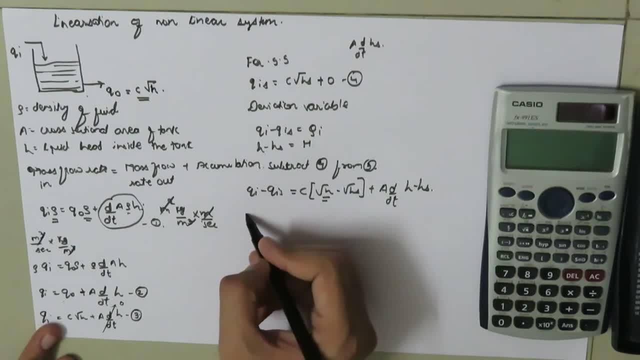 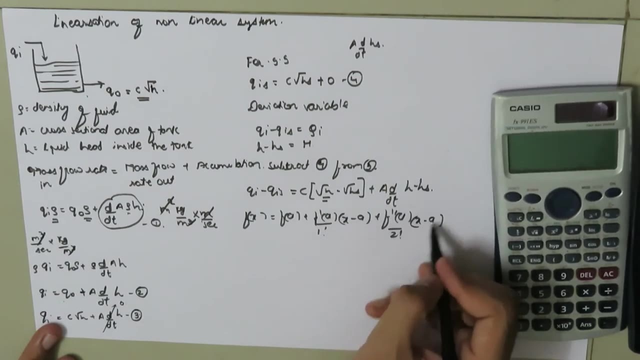 use of our Taylor series. so we know that Taylor series is: f x is equal to f a plus f dash a over one factorial times x minus a plus f double dash a over two factorial times x minus a square. but we are going to neglect the higher order derivative and we are going 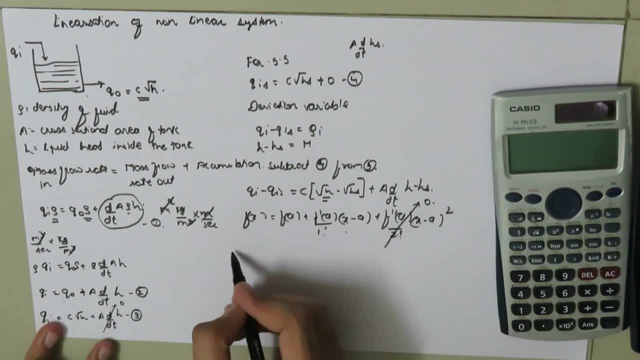 to consider only the, the first order derivative. so root H will be equal to root H s, plus one over two root H s. one factorial is one, so we only need to write H minus H s. let's call this equation number five. if you put equation number five in equation in this equation, so we: 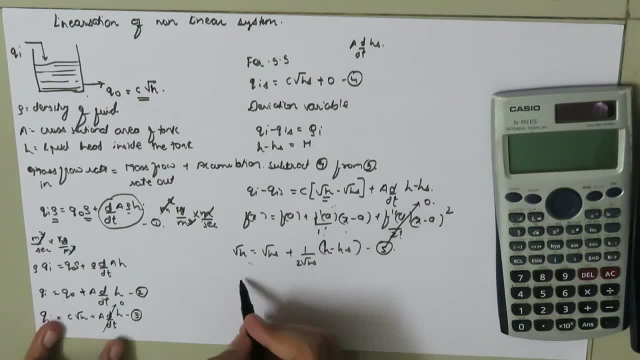 are going to substitute the value of root H as this, and this is our Q I minus Q s is capital Q I is equal to C inside the bracket: root H s plus one upon two root H s, times H minus H s. negative root H s as it is, plus a times D by DT of capital H. so this two term. 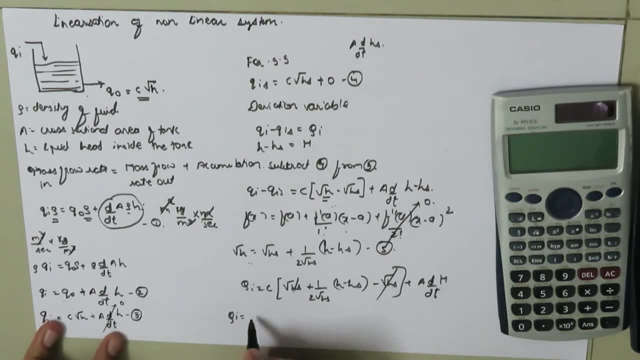 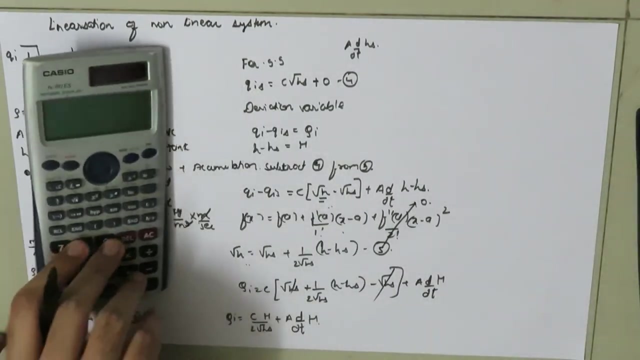 will get cancelled and we are left with Q. I is equal to C times. this can be written as capital H over two root H s plus a times D by DT of H. and now we are going to take the Laplace transform on both side of this equation. so if we take the Laplace transform, 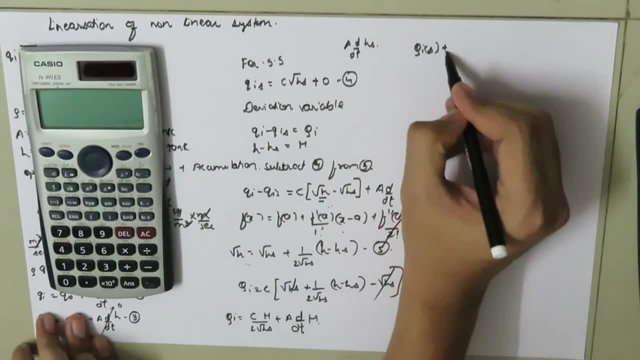 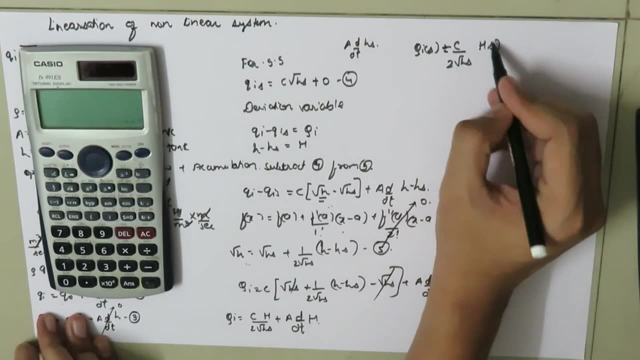 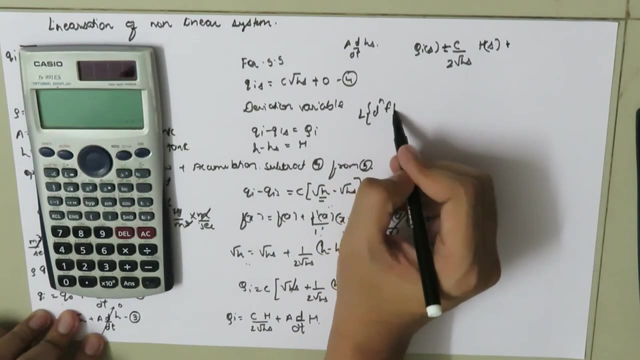 on both side of this equation. so this will be Q I s plus C O, which is equal to C over two root. H s is constant and H? s is negative. Now we know that the Laplace transform of D and F of T by DT n is equal to s to the. 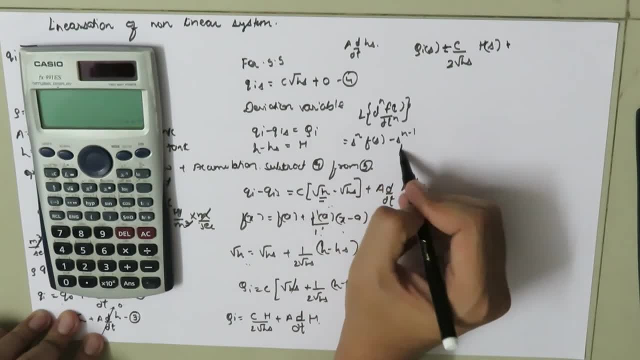 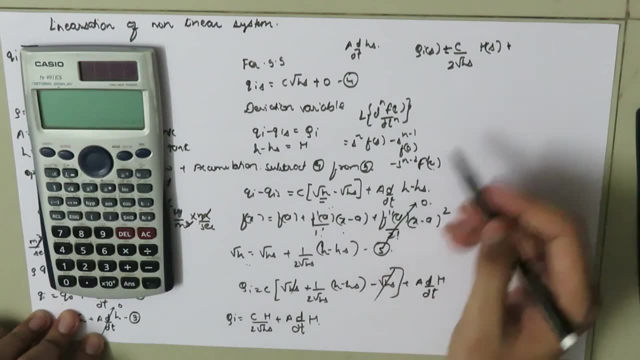 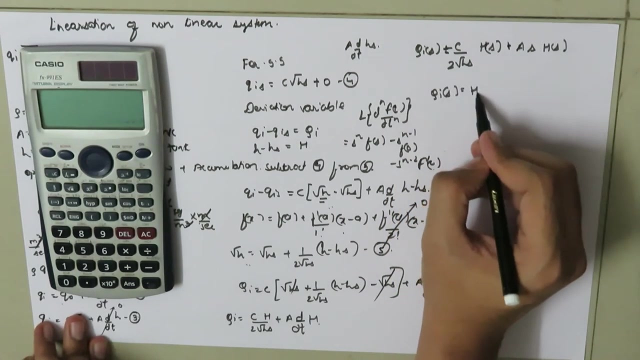 power n, F s minus s to the power n minus one, F zero. minus s to the power n minus two F dash zero. so this term as a constant. so this will be s times s to the power, one times H? s, And this will be Q. I s will be equal to if we take H s common from these two terms. so 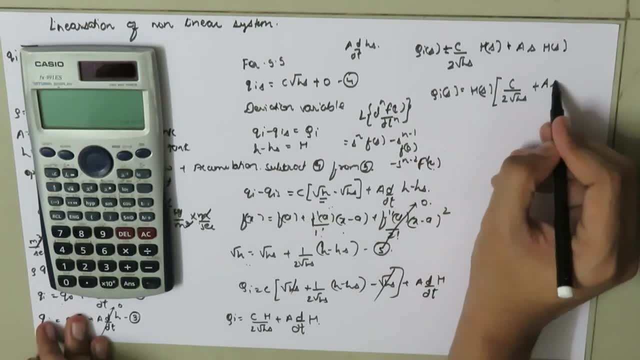 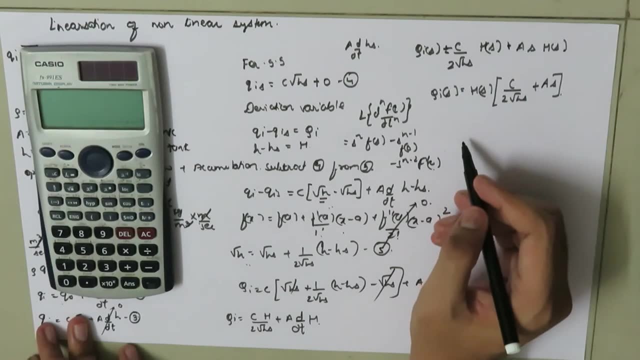 this will be C over two root H s plus a s. and now we know that the transfer function is in the form of the Laplace transform of output division variable divided by the Laplace transform of input division variable. so our output division variable is H, s and the Laplace. 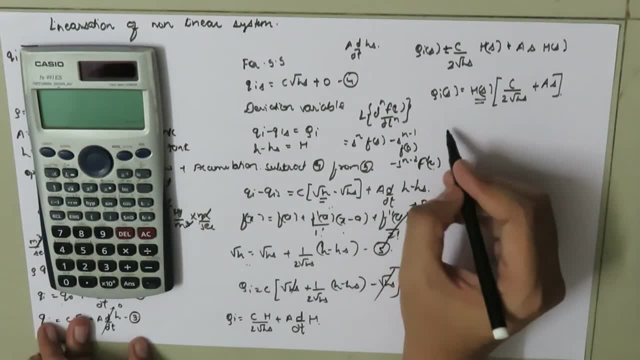 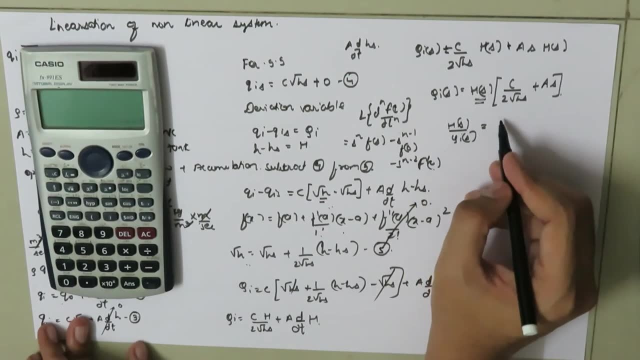 transform of input division variable is H s, So this will be a test over Q I s will be equal to 1 upon C upon two root H s plus a s. If you simplify this term, we get one upon C plus two root H s is over two root H s, and. 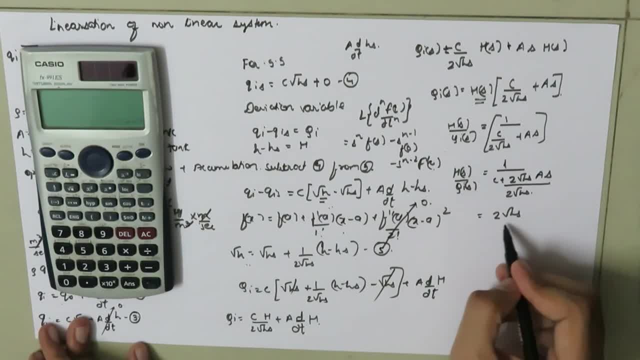 edges, and this will be true edges over C plus 2 root edges times. yes, and now we are going to compare this transfer function with our standard first order transfer function, which is in the form of: so, in the case of the standard first order transfer function, it is in the form of R upon 1 plus tau s. so we are. 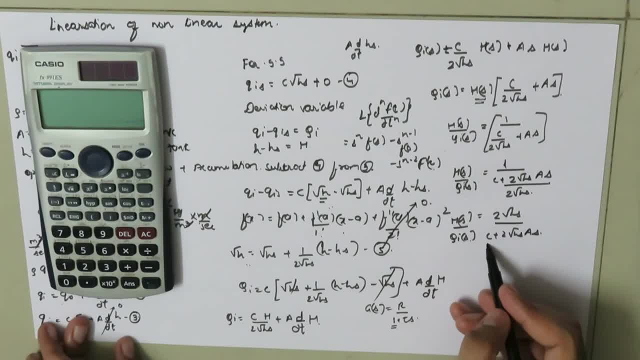 going to make this term. 1 means we had, we have to take C common, so true root edges upon. if we take C common, this will be 1 plus 2 root edges times a, divided by C times s, and this can be written as 2 root edges by C over 1 plus 2 root edges. 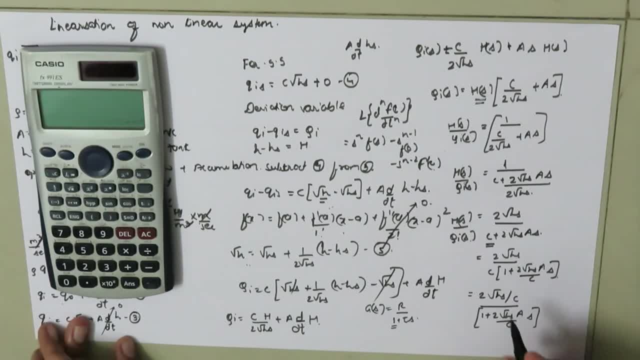 times a by C multiplied by s. and if you compare this equation, this is our transfer function- edges over Q is: if you compare this transfer function with the standard first order transfer function, then it is very clear that our time constant tau is 2 root edges times the cross-sectional area divided by C. so this is the transfer. 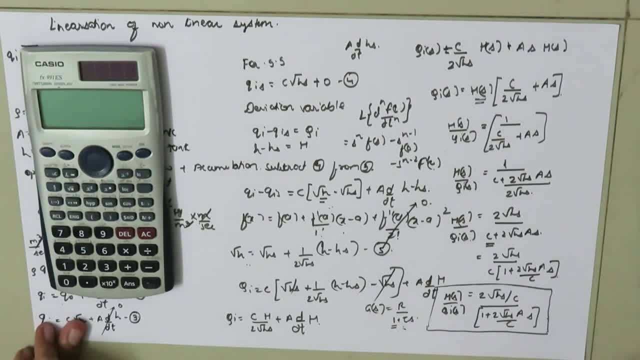 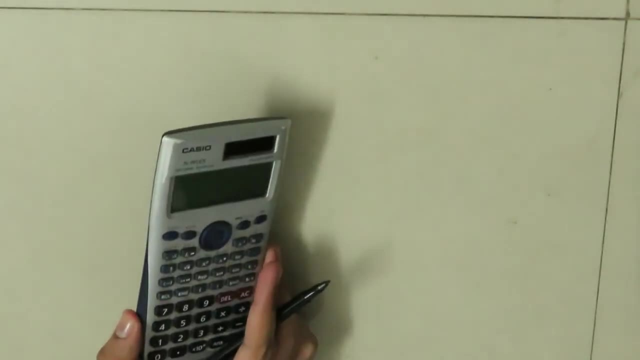 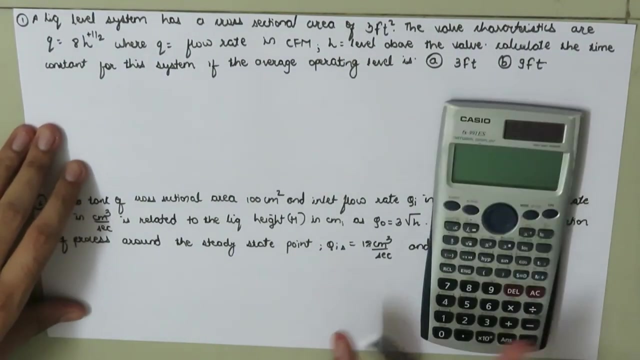 function in the case of linearization of the nonlinear system. and now, in order to get the deep understanding of this transfer function, we are going to solve two problems which are dependent upon the linearization of the nonlinear system. and now here we have our first example: liquid level system has the 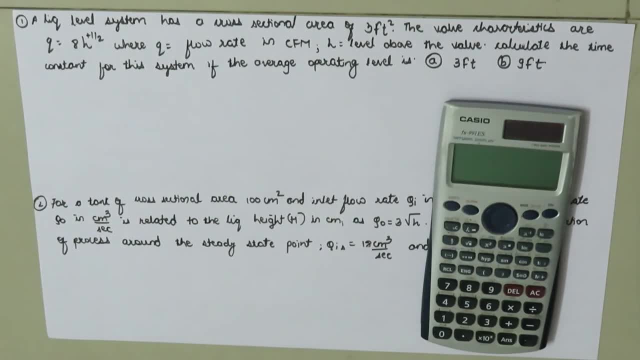 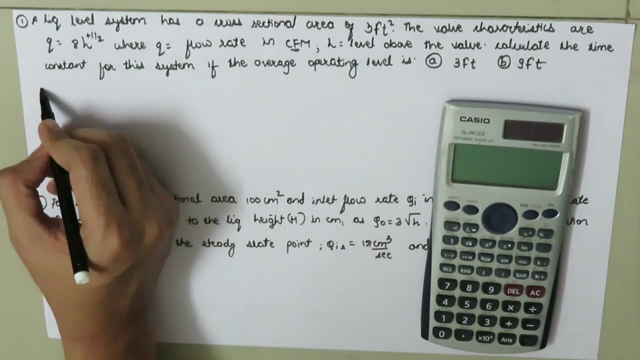 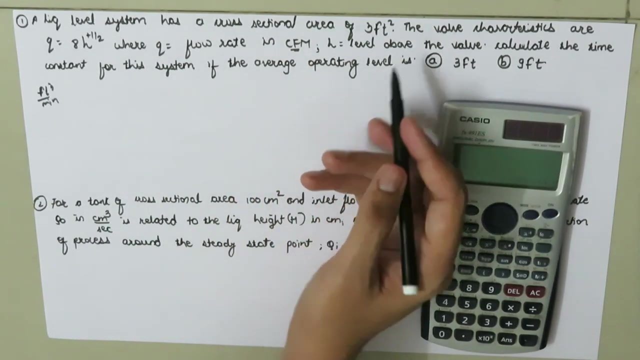 cross-sectional area of 3 cubic feet, the value of the measured ou three feet square, the value of the shaft Serv 來 per minute, that is, in feet cubed per minute. this term CFM and H is the liquid above the wall. calculate the time constant for this system if the average 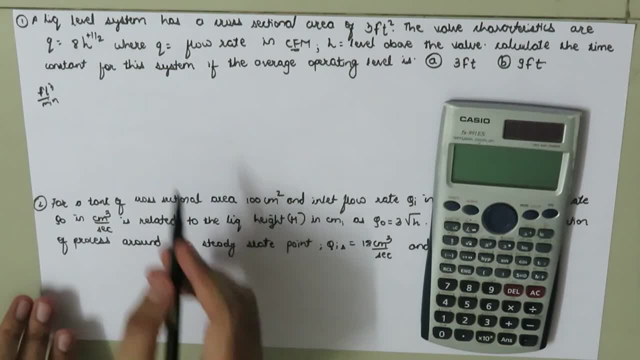 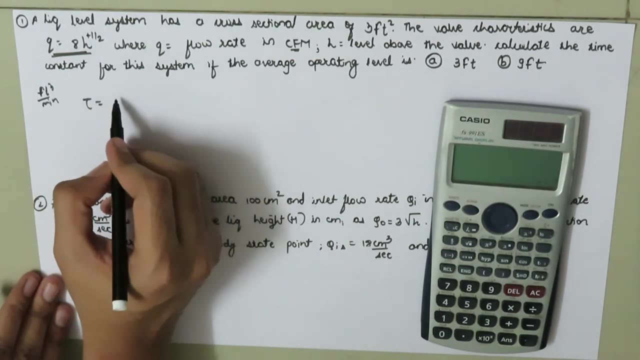 operating level is 3 feet and 9 feet. so we know that by looking at this expression, we should easily identify that this problem is related to the linearization of nonlinear system. and in the case of the linearization of the nonlinear system, we derived that our time constant tau is equal to 2 root hs. 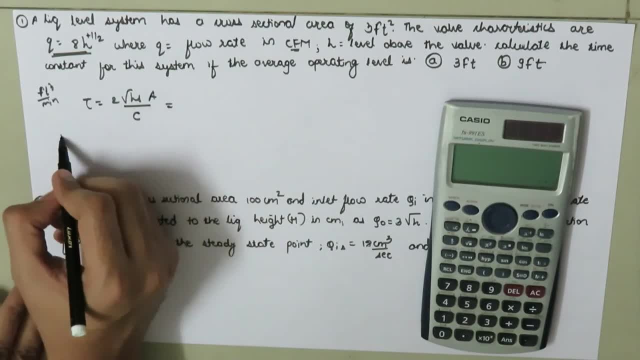 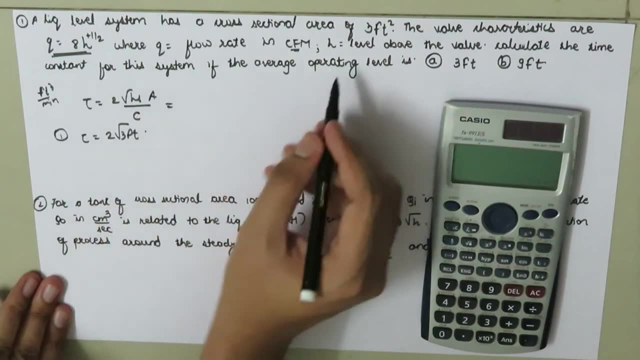 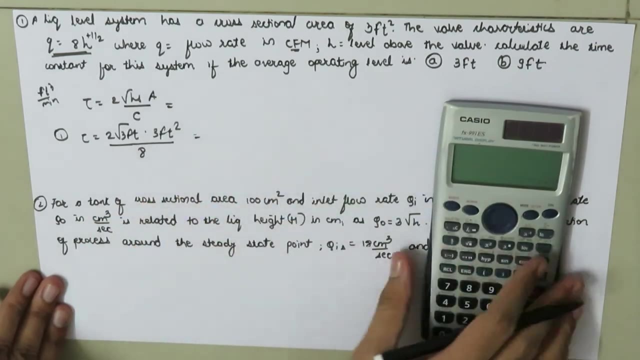 times a by C. so in the first case our tau will be equal to 2 root. hs is 3 feet times our area is 3 feet square divided by, instead of C, here we have 8, so this will be our 2 root 3. 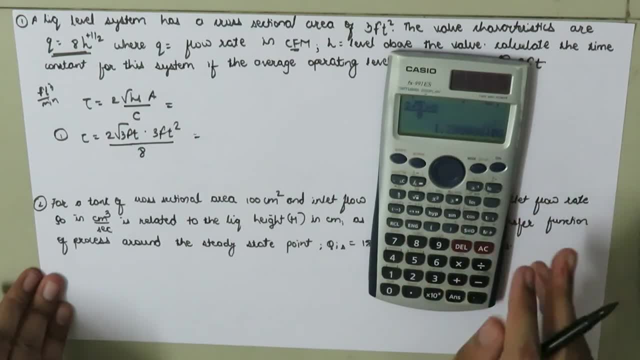 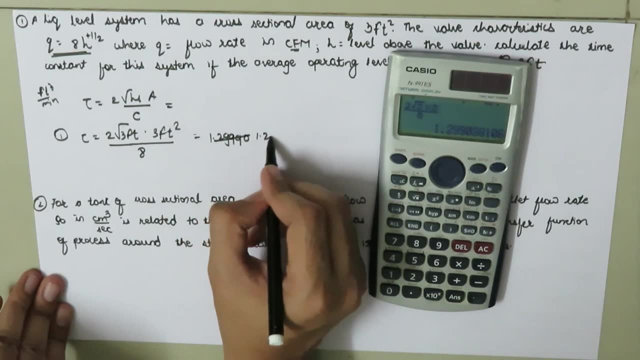 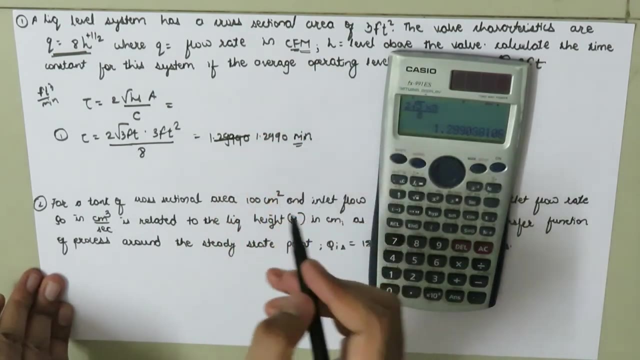 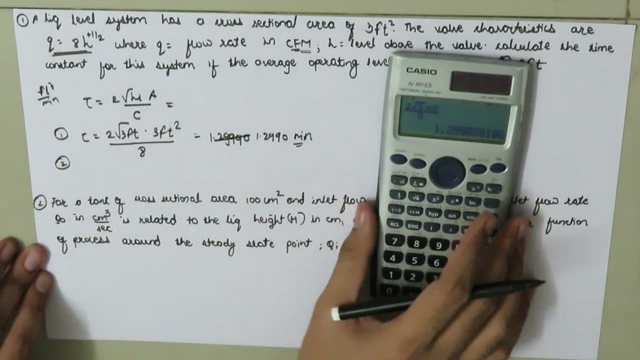 multiplied by 3, divided by 8, so your time constant will be one point two, nine nine zero. this is one point two, nine nine zero minutes because our flow rate is in minutes, so our time constant. our flow rate is in cubic feet per minute, so our time constant. and in the second case we are gonna take the root H as 9 feet. 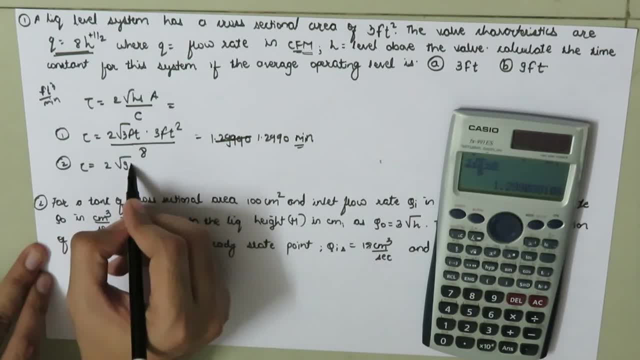 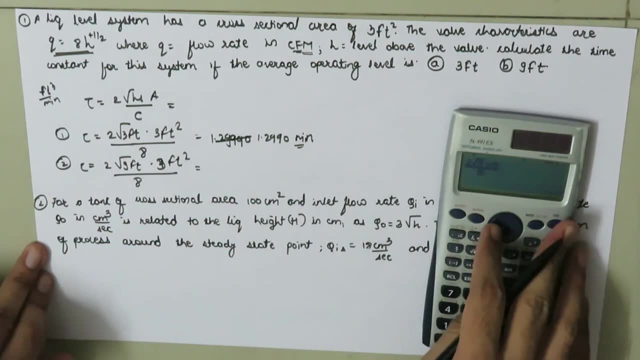 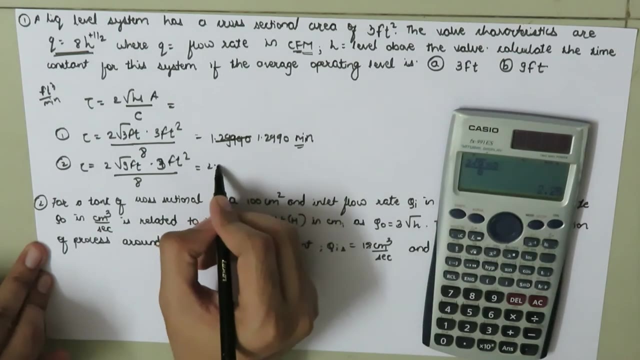 so tau will be equal to two root hs times 180. your control will stop the rotation. replacement to the önlaus: 당신까지 인 vac yogurtat. two root nine feet times three feet square over eight, so this will be 2.25 minutes.